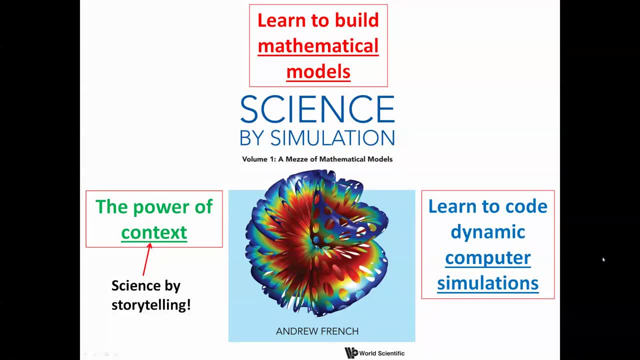 context. Learn techniques because you have to understand a story, be it the epidemiology of EAM, Descartes' model of a rainbow, the atmosphere, strange, chaotic attractors of modelling, stock trading or indeed elections. Number three: build computer simulations yourself. Make the. 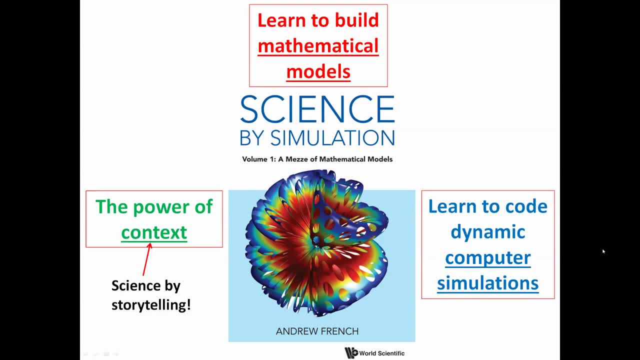 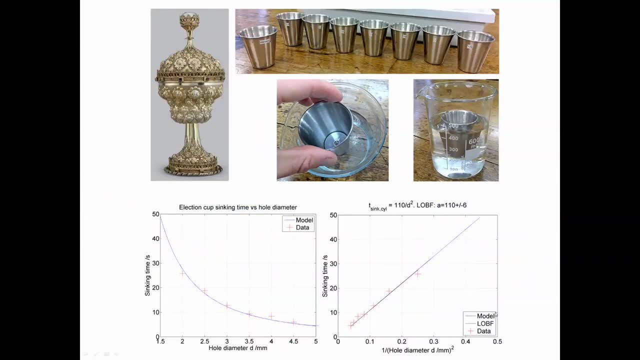 bridge between reality and abstract, problem solving and develop creative skills that will make you useful as a scientist. So, introductory chapter, an example of an experimental analysis process via election cups. The time it takes a cup to sink varies as the inverse square, as the diameter of the hole drilled in the base of the cup, And we can do lines of best fit and follow. 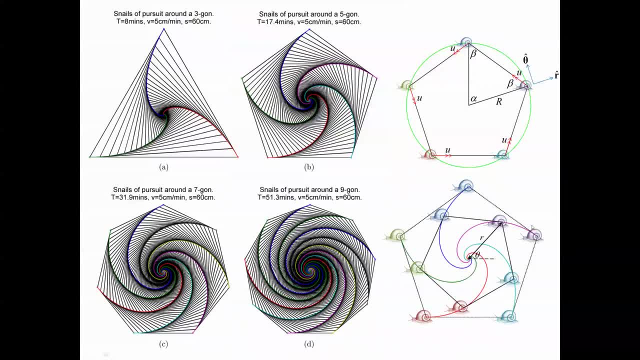 the data processing pipeline. as a result, Snails of pursuit can only move at fixed speed, but can change direction. A powerful gastropod pheromone causes them to chase each other. Their initial polygon arrangement will therefore rotate and contract until the snails meet in a 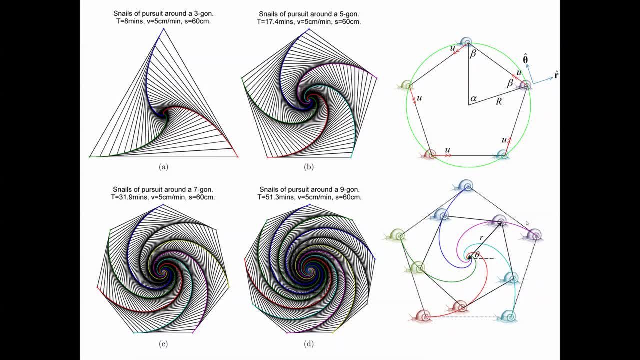 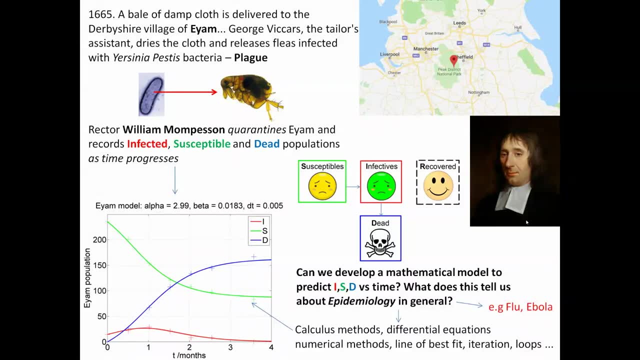 writhing slimy mess. This is an example of a mathematical modelling and, importantly, the importance of visualisation. Now, in 1665, the plague devastated the Derbyshire village of EAM. The rector, Winwin Mumpasson, kept accurate parish records of those infected. 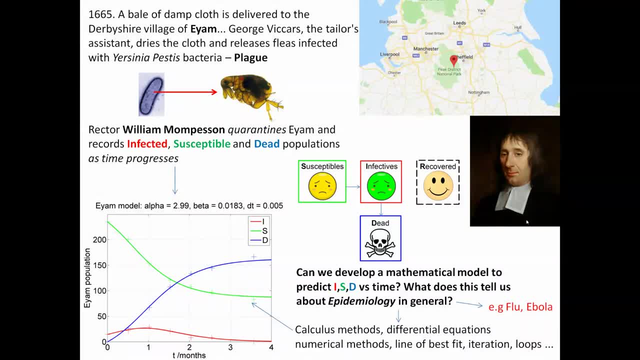 susceptible and those that had died. Plot and model these ISD curves with time and you have the basis of the science of epidemiology. This is the largest chapter of science, plus simulation, and we apply the EAM equations to Ebola and indeed, in a certain restricted way, to COVID-19.. 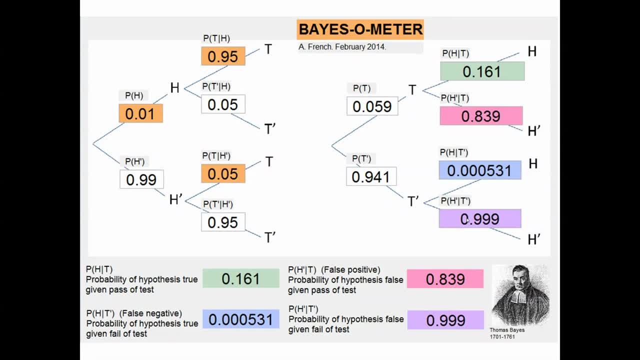 Bayesian inference, ie the probability of a hypothesis being true given observational data, is one of the most important ideas of science. The Bayesometer demonstrates how probabilities can be unexpectedly low if the hypothesis is rare and tests are not perfectly accurate. May's bivocating bunnies model of rabbit population. 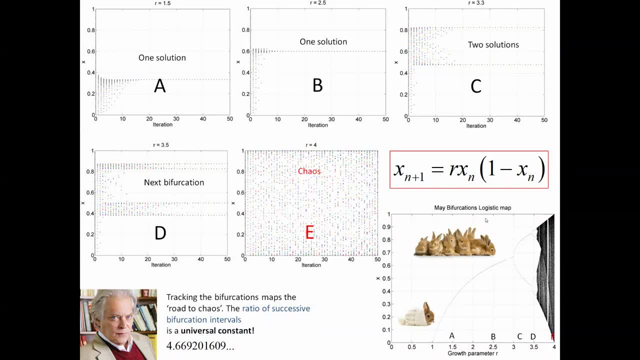 which is a classic gateway to chaos theory ideas. The maximum population fraction next year, X, depends on this year's population fraction. Depending on a growth parameter R, the asymptotic population either crashes, stabilises, oscillates or indeed becomes entirely chaotic. The double pendulum is an example of a mechanical system that can become chaotic. 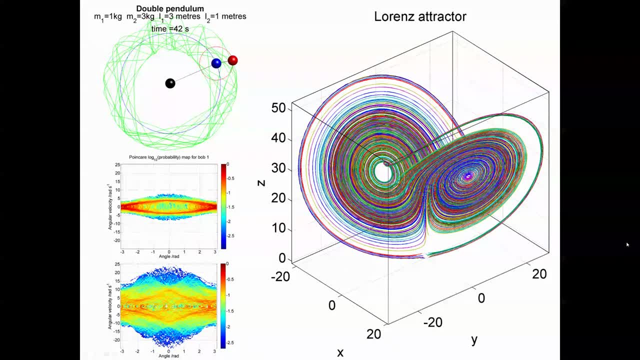 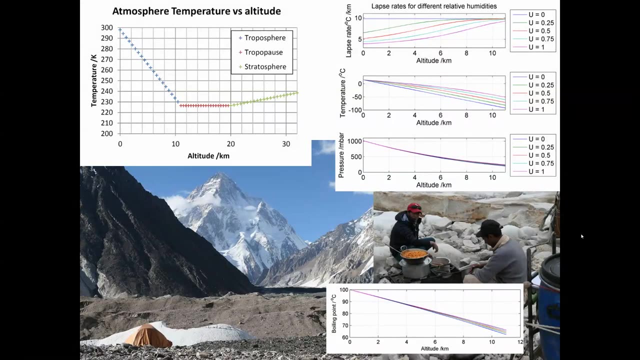 Conversely, Lorenz's system of weather predictions produces a strange attractor, a butterfly-shaped region of the parameter space X, Y and Z that vary with time, t that all time histories appear to gravitate towards. A model of the atmosphere is developed and temperature pressure boiling point, and 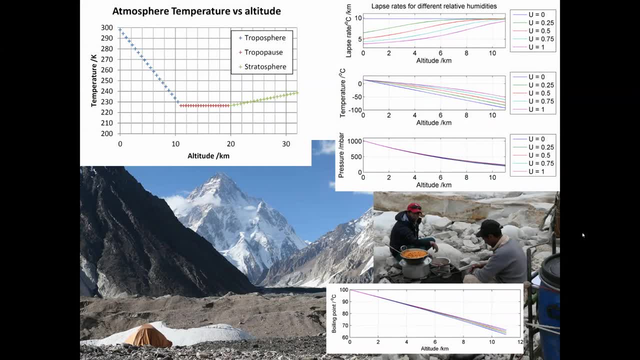 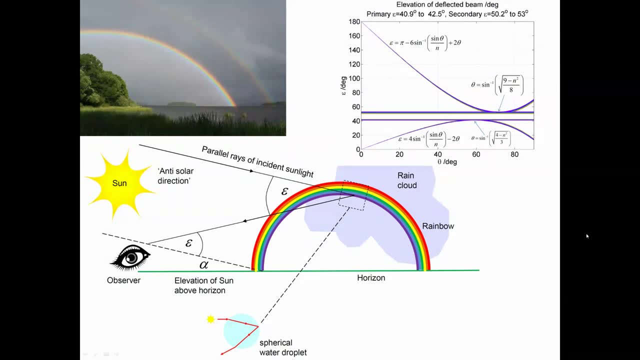 elapsed rates are predicted versus altitude for varying levels of humidity. Descartes' model of a rainbow, incorporating the subtle variation of the refractive index of water with the wavelength of light, allows us to predict the elevation of primary and double rainbows from. 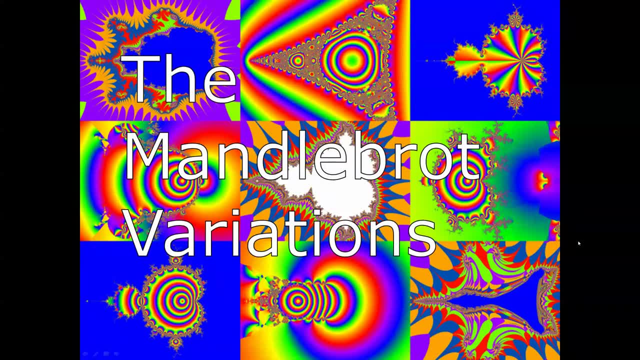 the direction of the sun. Organic-looking fractals of Benoit Mandelbrot are generated from very simple mathematical recipes involving complex numbers. In addition to the classic beetle-like picture, we can create light bulbs, rockets, plants and bacteria-like forms. 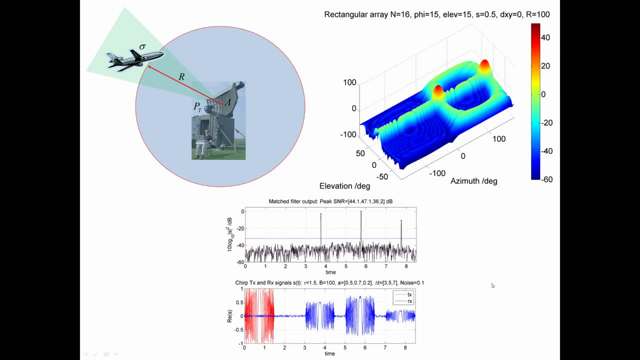 and indeed Buddhist imagery. I will have three concepts of radar: how to work out the signal-to-noise ratio with range, how to steer a beam of microwaves electronically via a phased-array antenna. and how to improve range resolution by transmitting frequency-coded pulses, Starting with Eratosthenes and Al-Biruni's methods. 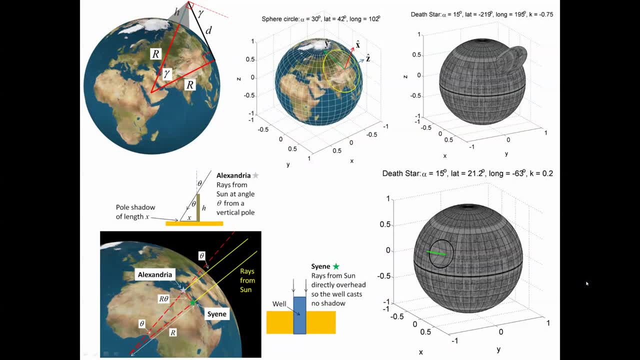 we shall navigate the sphere and explore the ancient techniques of geodesy. How far is the horizon? How can we measure the radius of the Earth using weights, some string and a protractor from the summit of a mountain, And indeed, how we can plot the Death Star. Can we make sense of 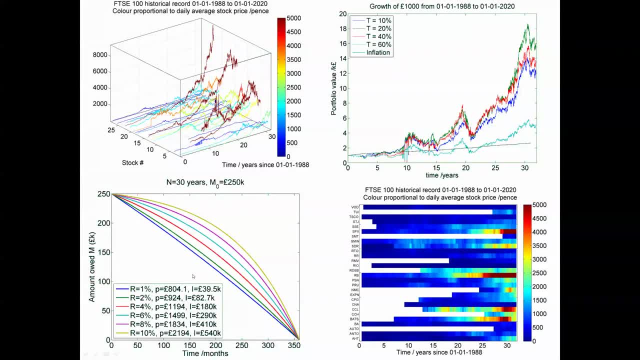 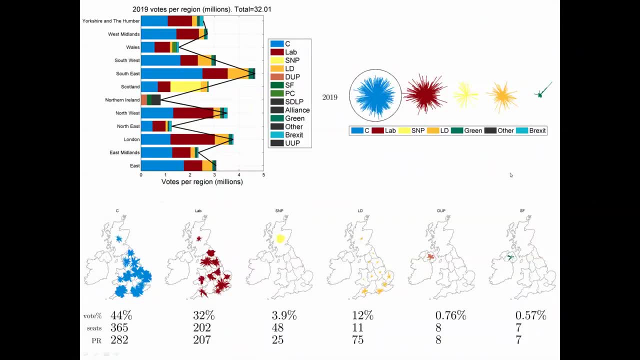 money. Can we make sense of money? Can we make sense of money? We shall study philosophical mortgages, savings schemes and virtually dabble in stock trading. Finally, in Power to the People, the concluding chapter, we shall analyze recent UK General 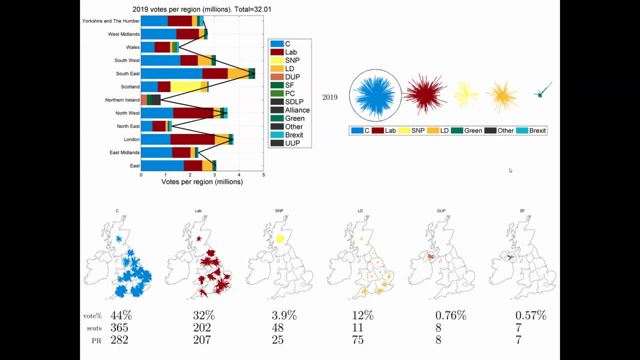 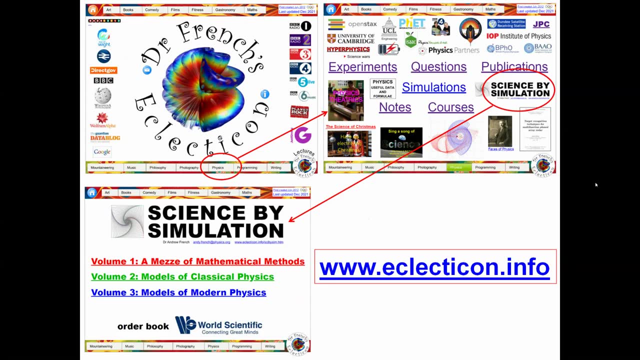 Elections. Were they fair? What could be the unintended consequence of a proportional system being? Could we model the details of how it might work in practice? Science by Simulation is available to purchase from the World Scientific Online Bookstore. You can access it by my eccentric